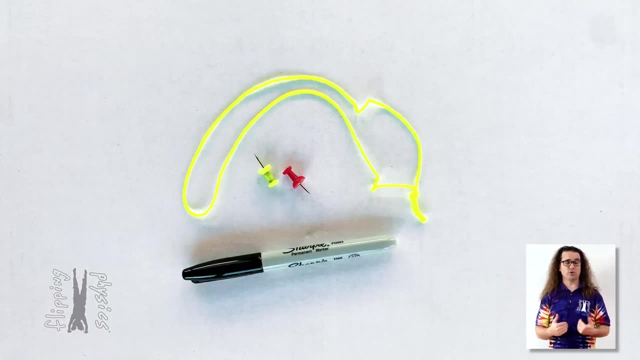 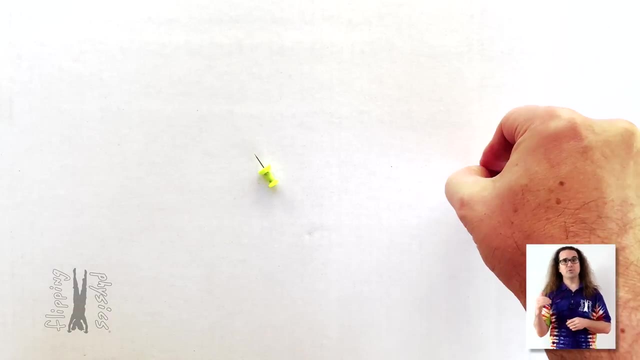 Well, we're going to start with a conclusion based on observation. Absolutely, Yeah, sure, Alright, Let's draw an ellipse. We start with a piece of cardboard, two thumbtacks, a piece of string tied in a loop and a writing utensil. We can place the two thumbtacks. 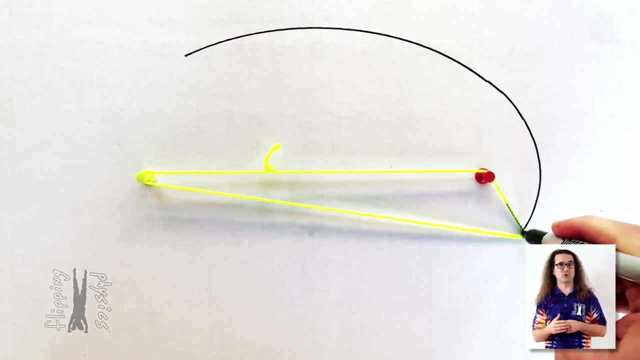 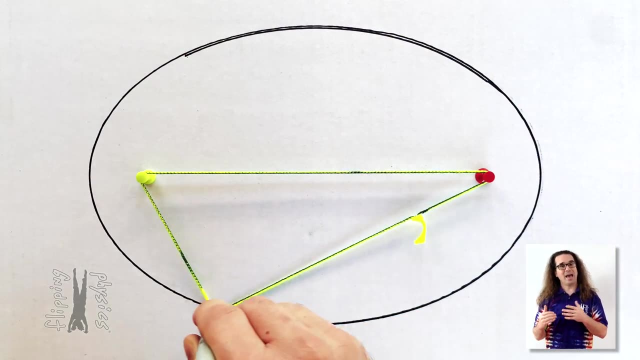 which become the foci of the ellipse. And by looping the string around the two foci we can use a marker along with the looped string to draw an ellipse And then redraw the ellipse to make it darker. And there you have it, An ellipse with the two foci where the thumbtacks are. 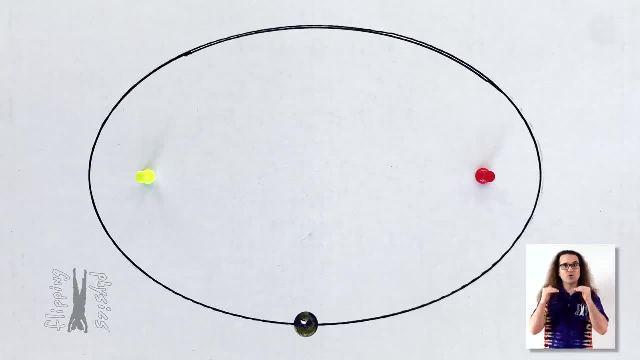 This represents the elliptical orbital paths of all satellites. where the satellites follow the path of the ellipse, The central body or the object the satellite is orbiting is located at one focus and there is nothing located at the other focus. And now let's switch to a more accurate ellipse I used the computer to create. 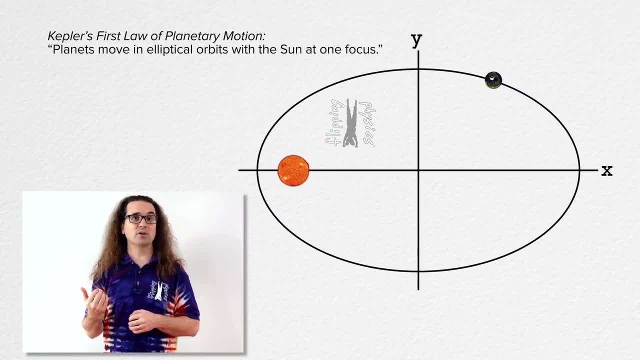 I have added an x-y coordinate, A coordinate system, to help identify parts of the ellipse. The two foci are labeled f sub 1 and f sub 2.. The elliptical curve is drawn such that the sum of r sub 1 and r sub 2,. 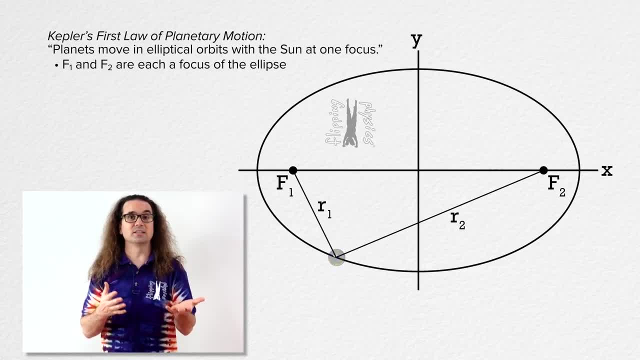 the distances from the respective foci to the elliptical curve is constant. In other words, r1 plus r2 equals a constant number. That was the purpose of the string. That is how we physically made r1 plus r2 equal a constant number. 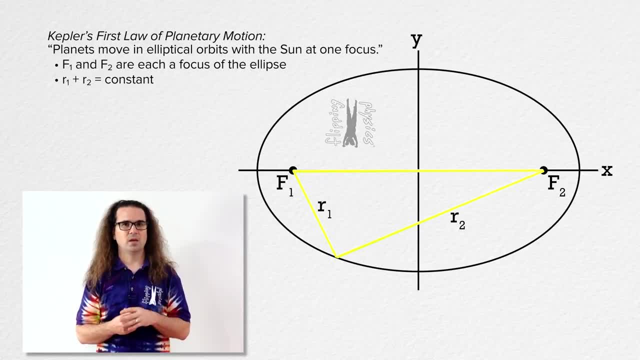 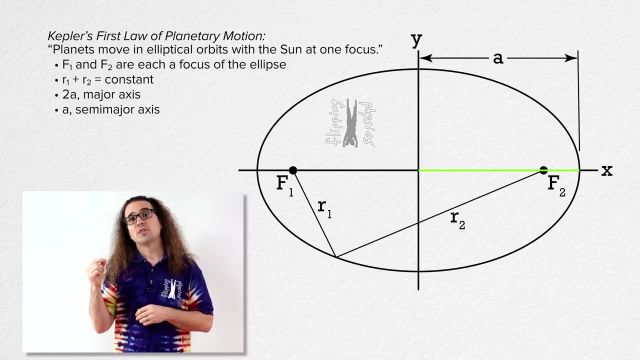 because the length of the string was constant. The major axis is the longest distance through the center, which also passes through both foci, and is the distance 2a, where the distance a is called the semi-major axis. The minor axis is the shortest distance through the center. 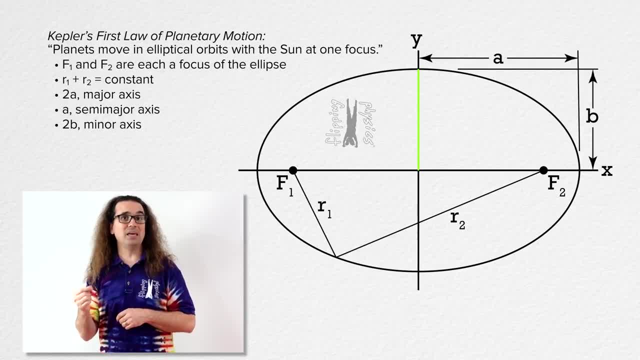 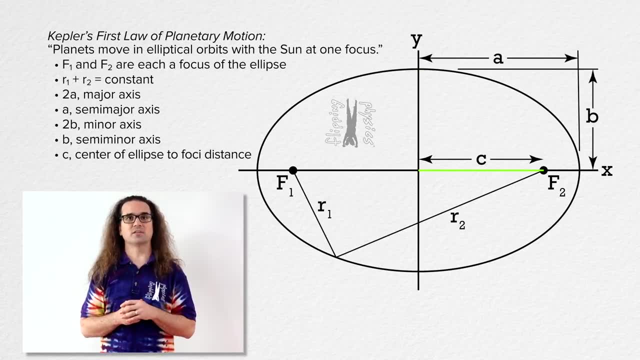 and it is the distance 2b. where the distance b is called the semi-minor axis, Each focus is located a distance c from the center of the ellipse. Unfortunately, not all textbooks agree on which letters to use for these distances in an ellipse, so 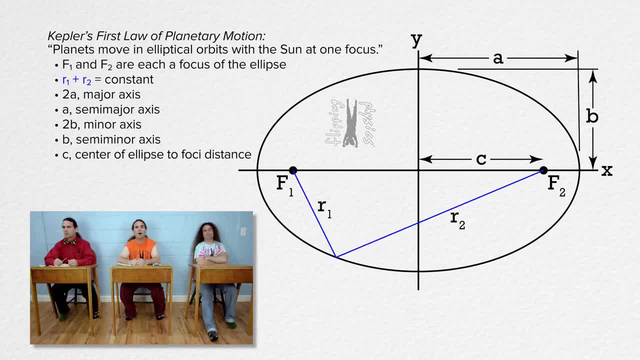 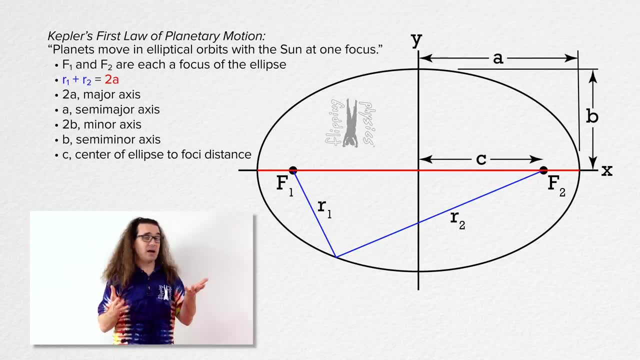 Fun, Yeah. So r1 plus r2 equals the major axis 2a, Right, Mr P Billy? that is correct. Now that we have defined the major axis, we can identify that the sum of the two distances from each focus. 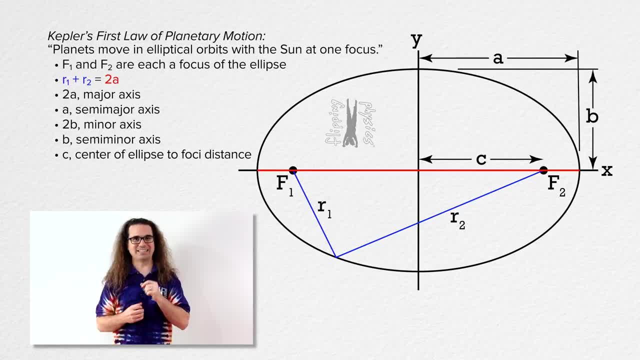 to any point on the ellipse equals the major axis. I also want to point out that at the location where the ellipse intersects the y-axis, the two distances from the foci to the ellipse are equal in value and are also equal to a, the semi-major axis. 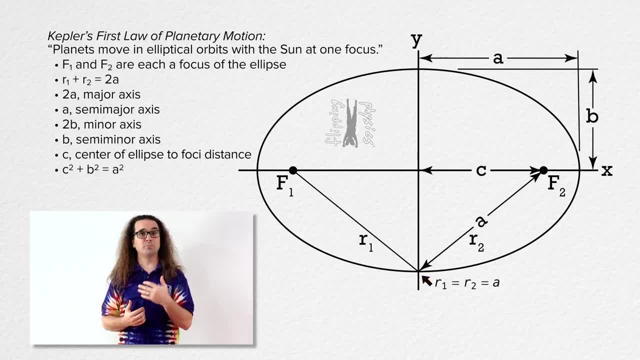 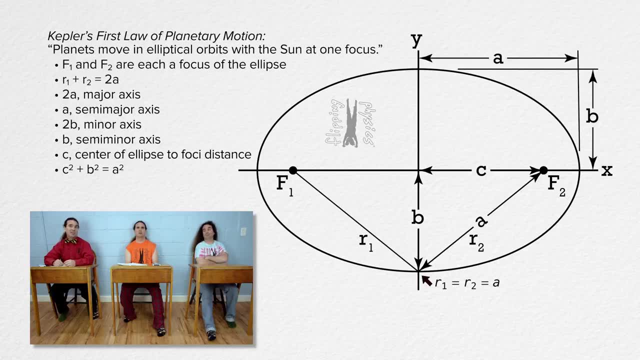 That means for an ellipse, c squared plus b squared equals a squared. I thought a squared plus b squared equaled c squared. This is not the Pythagorean theorem, It is the definition of an ellipse. Those are two different things. 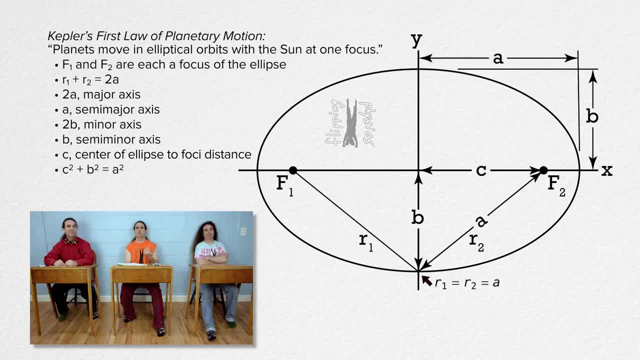 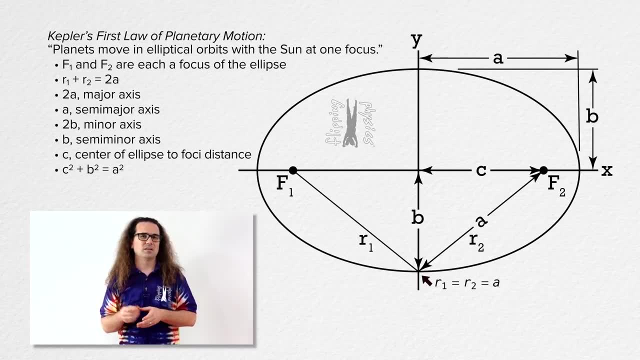 They sure look similar. Yeah Yeah, that is unfortunate. For an ellipse, c squared plus b squared equals a squared. Let's define the eccentricity of an elliptical orbit. Eccentricity lowercase e equals c- the distance from the center to one focus. 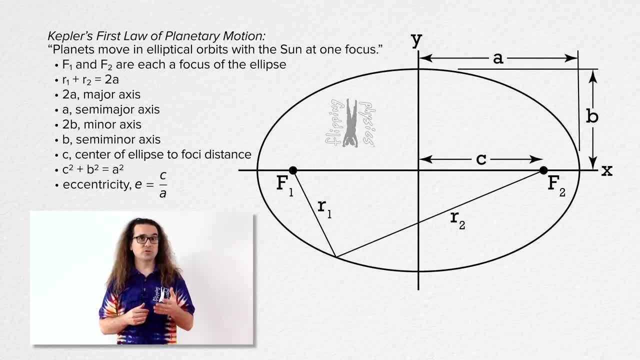 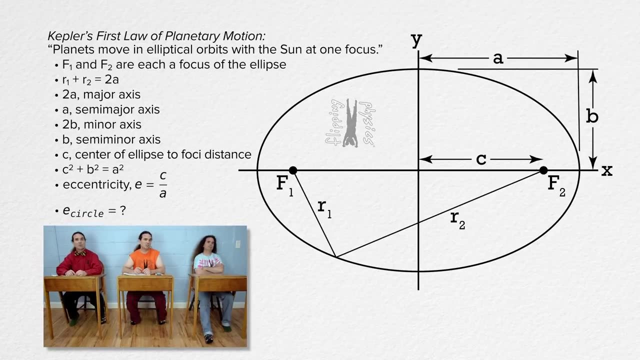 divided by a, the semi-major axis. Eccentricity basically describes how circular an ellipse or an orbit is. Bobby, what is the eccentricity of a circle? The eccentricity of a circle? Well, for a circle, the distance c equals zero. 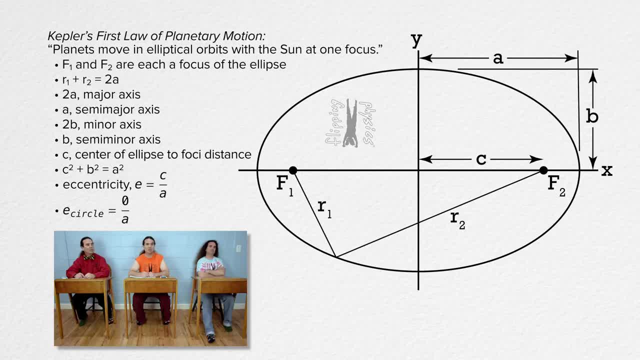 because the two foci are both in the same location, in the middle of the circle. That means the eccentricity of a circle equals zero over a or zero Correct. The eccentricity of a circle equals zero And if c equals a. 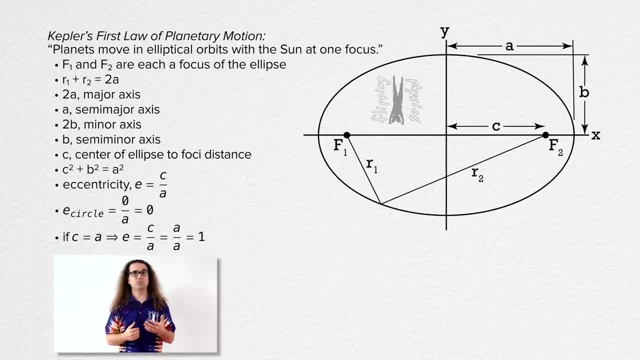 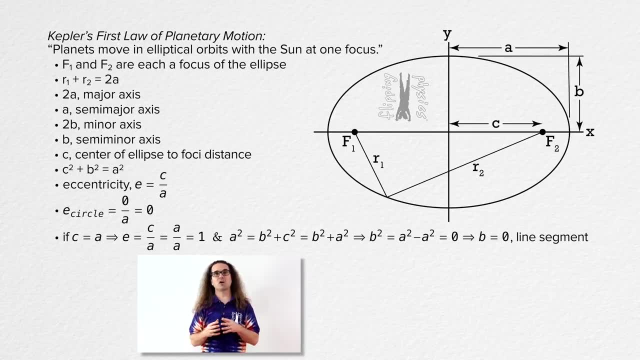 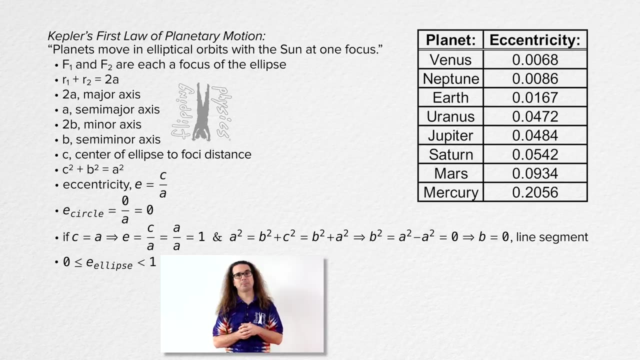 is an eccentricity of one, then b equals zero and the ellipse is actually just a line segment. Therefore, the range of eccentricities for an ellipse are between zero and one. And here are the eccentricities of all eight planets. I miss Pluto. 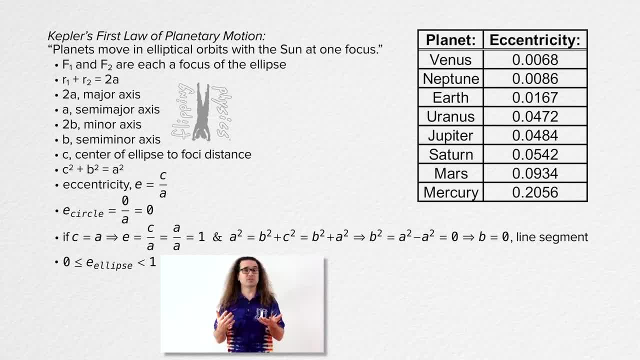 As you can see, the planet with the largest eccentricity is Mercury, at 0.2056.. To understand what an ellipse with an eccentricity of 0.2056 is, this is what 0.2056 looks like. this is a circle.